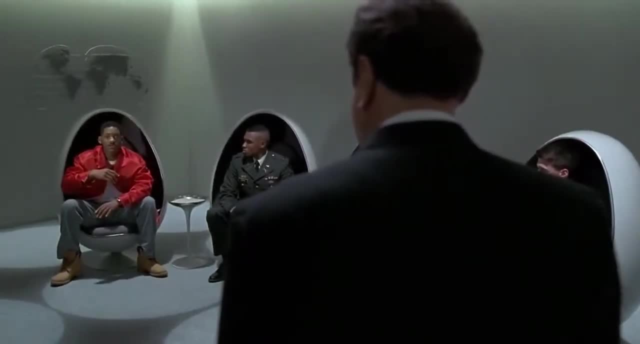 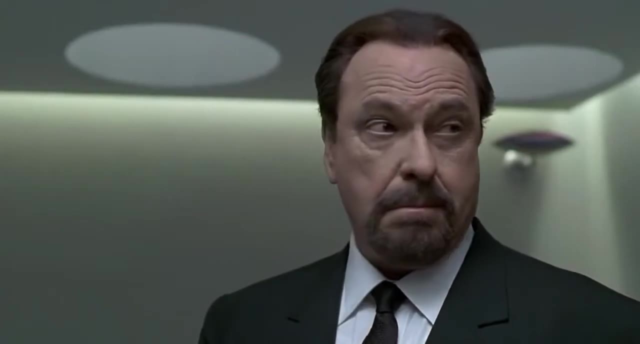 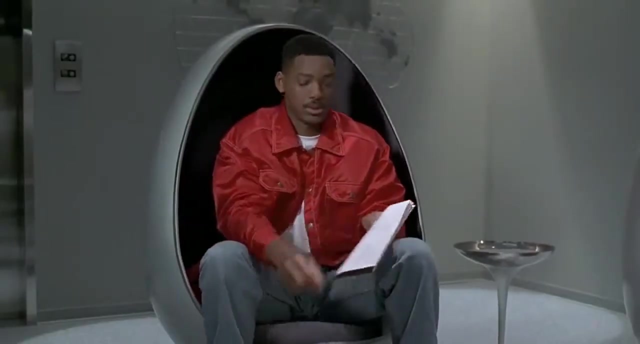 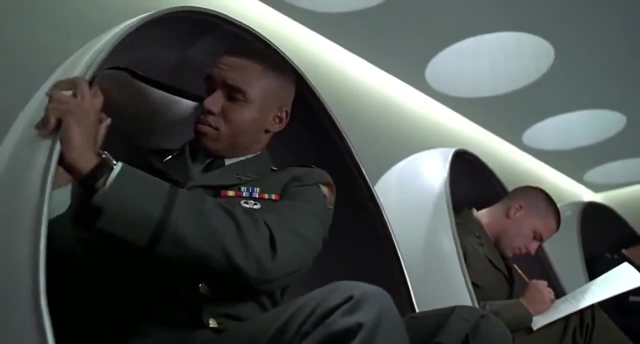 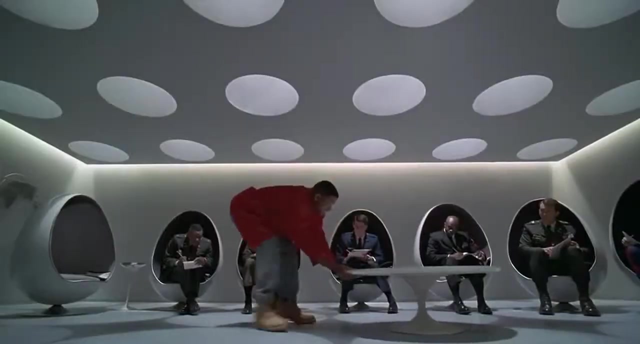 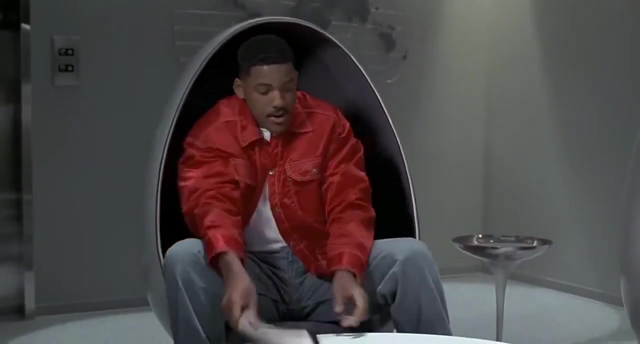 we have a question. uh, yeah, i'm. i'm sorry, maybe you already answered this, but uh, why exactly are we here, son? we're here because you're looking for the best of the best of the best. let's get going. do you want to get down on us? 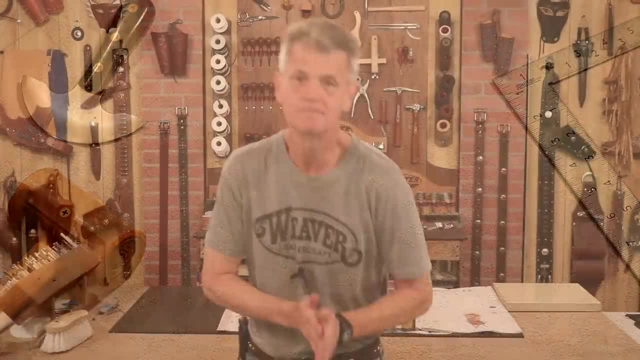 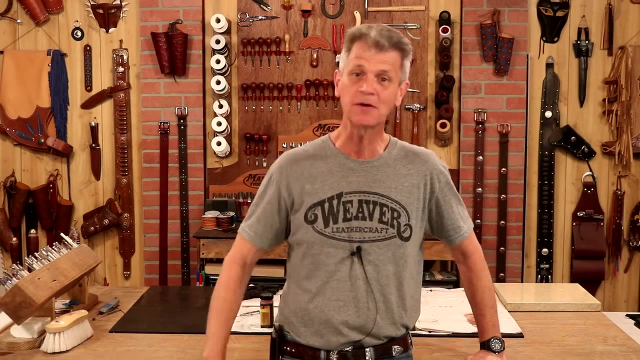 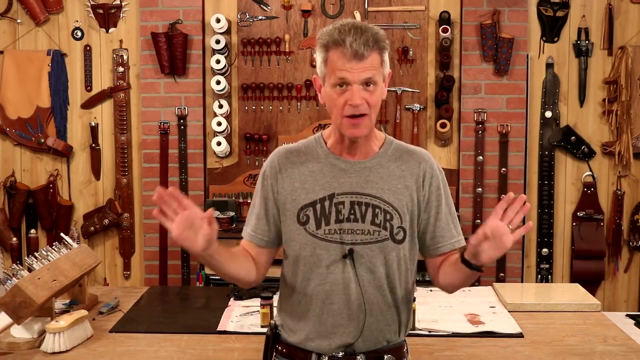 Hi, I'm Chuck Dorsett for Weaver Leathercraft and this is the Leather Element. If you've got a good question for us or a good idea for a Leather Element, drop it in the comment box below. If you've seen any of our videos, you know that I use Pro-Dye and nothing else. It answers all of. 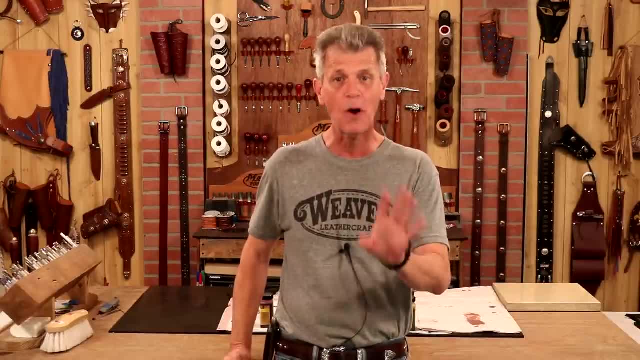 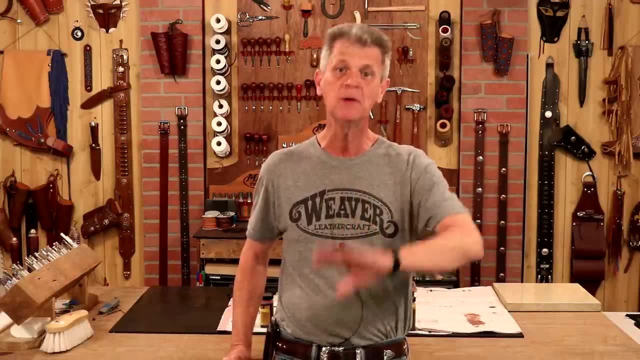 the issues I have with dyeing. But we get a lot of questions on water-based dyes, our leather colors. So let's take a look at these. But let's take it a step further. Let's do a comparison between the water-based dye, our leather colors and our Pro-Dyes. Let's see what happens And in 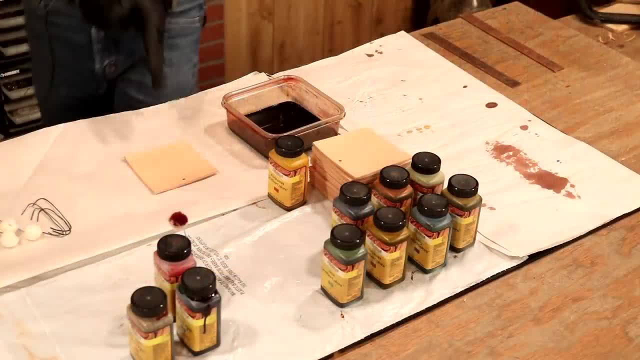 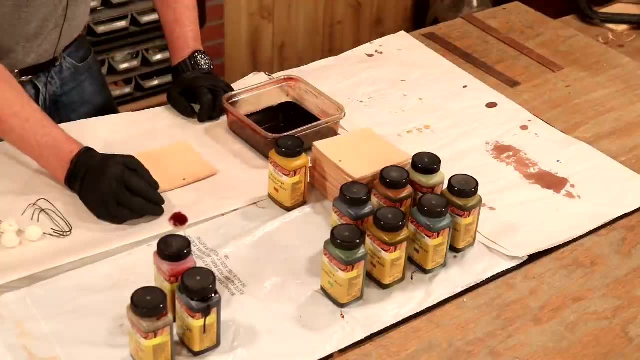 fact, I think I'm going to be surprised. Without making this overly complicated, we're just going to do this in a couple of simple steps. So, first off, I'm going to dip-dye all eight leather colors. Secondly, I'm going to dip-dye just a couple of Pros, so we have a good comparison. 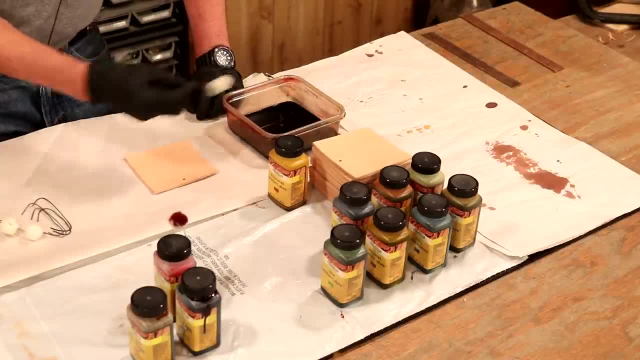 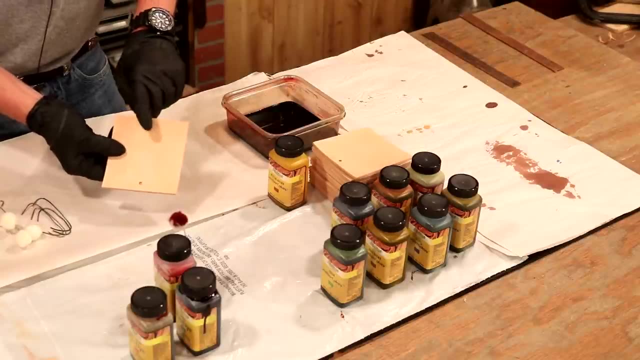 With a couple of swatches left over, I'm going to add the leather colors with a dauber. Let's just see how everything looks Now. right here I've got an 8-9. 9-ounce Weaver Select. It's going to give us a good color read, And with each diamond right on. 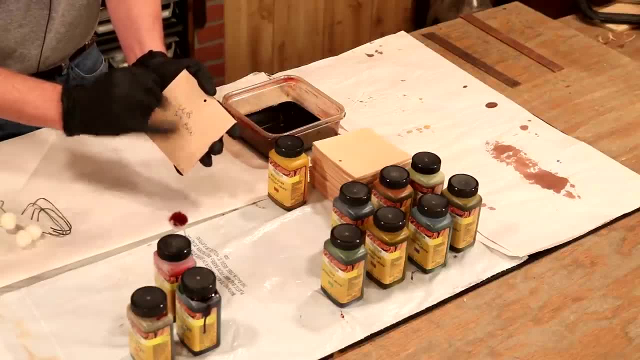 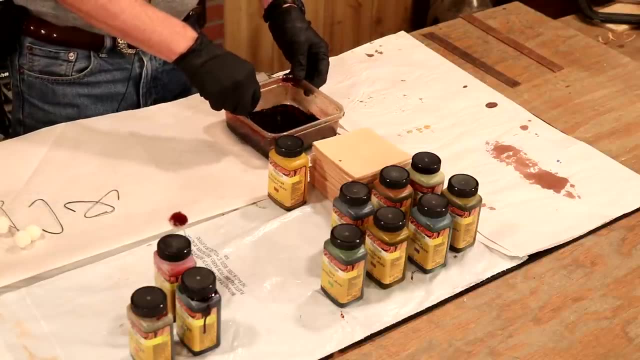 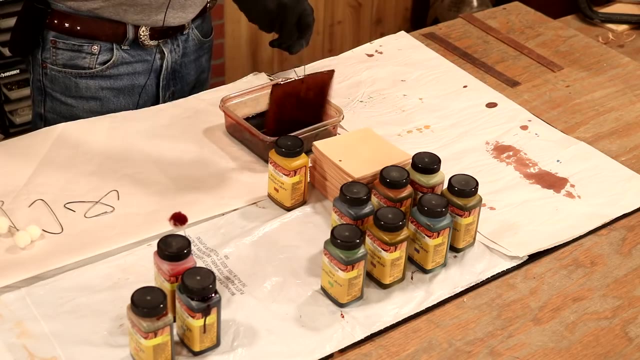 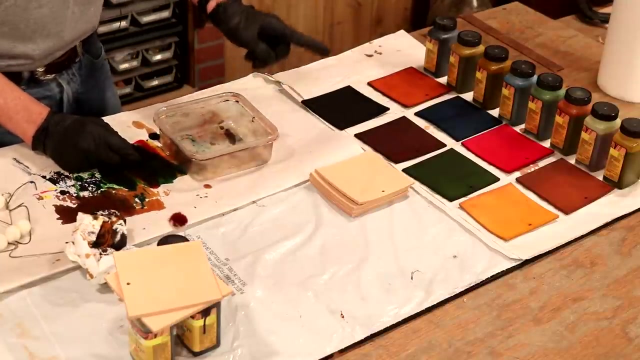 the back, whether we dip or dauber, what color, and whether it's water-based or Pro. Okay, our eight colors are done, Really happy with the outcome. Those are beautiful colors. Okay, going to dip-dye Same way. In fact, we're going to go with our Pro-Dye here We're.